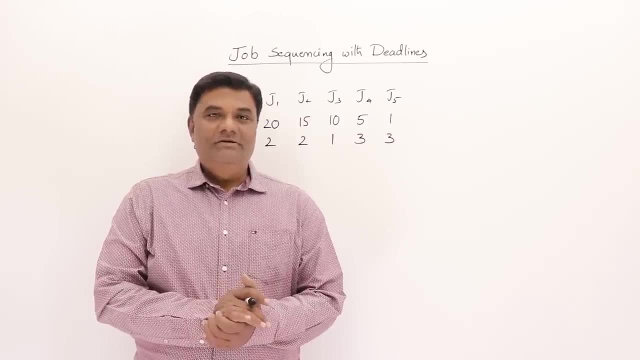 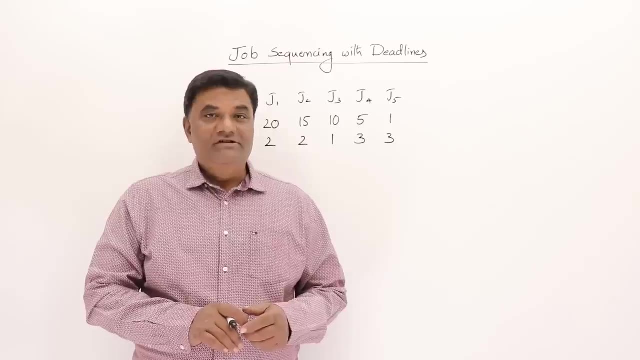 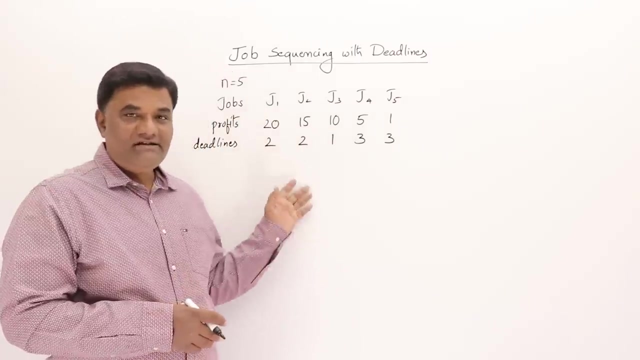 Hi. our next problem is job sequencing with deadlines. This problem we are going to solve it using greedy method. So first of all, we will understand what the problem is. Already, I have an example. Through an example, we will understand what the problem is, Then we will. 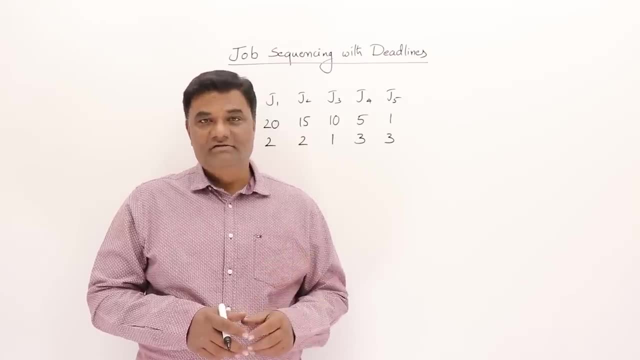 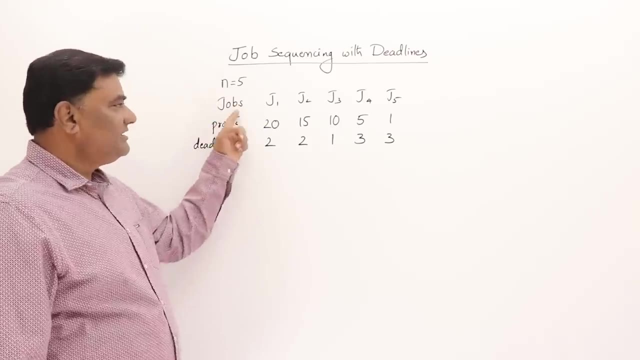 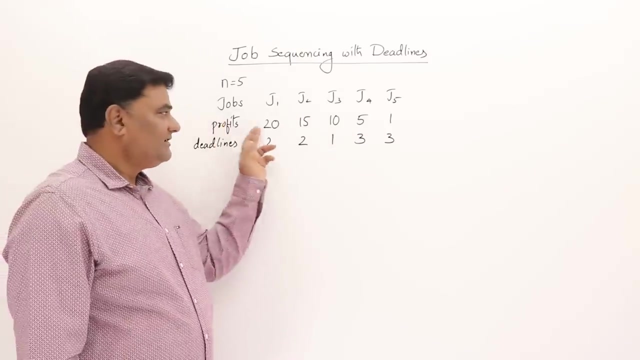 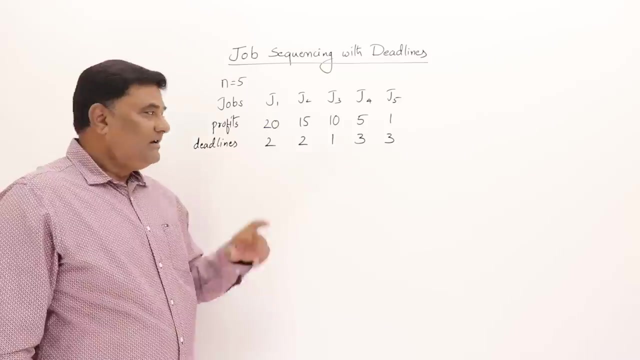 see how to solve it using greedy method. So let us know about the problem. See, here in example, five jobs are given, five tasks are given, and if that task is completed we will get this profit. So associated with each job there is some profit, But that job must be. 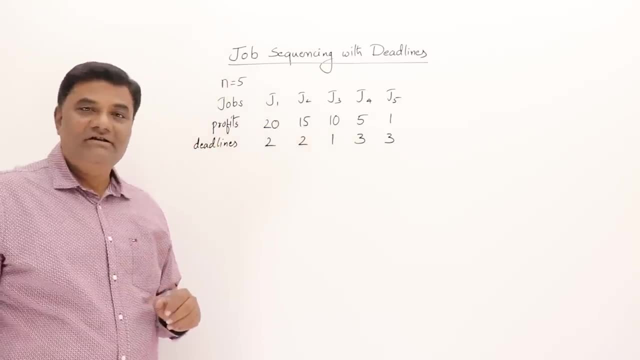 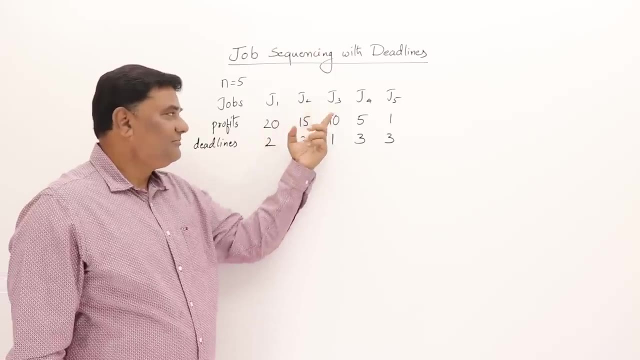 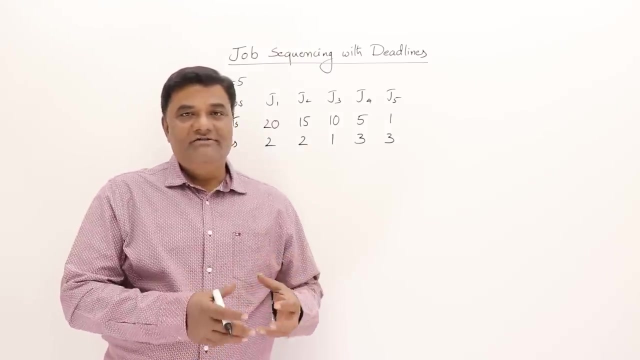 finished within this deadline. it must be completed within the deadline. Like first job should be completed within a deadline two and deadline. job two also two, job three is one. So like that, every job is having some deadline. So the problem is jobs are given, every job is having some profit and if you complete the job you will get the 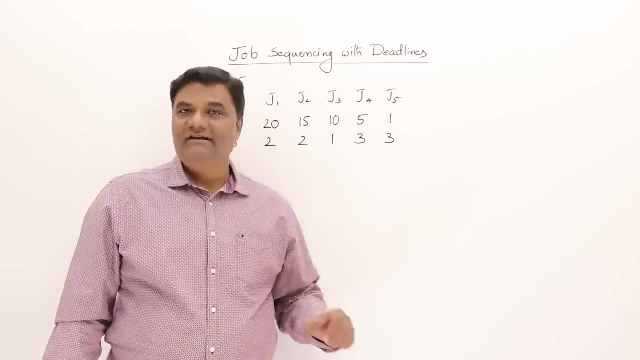 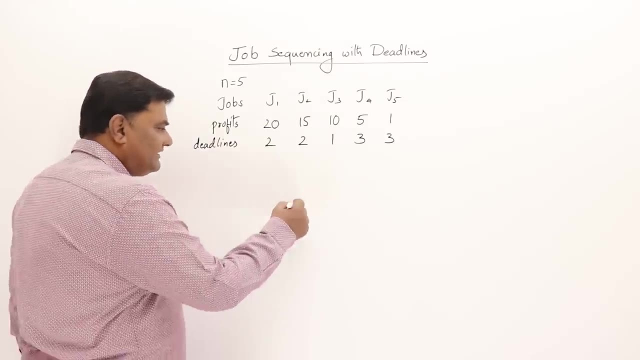 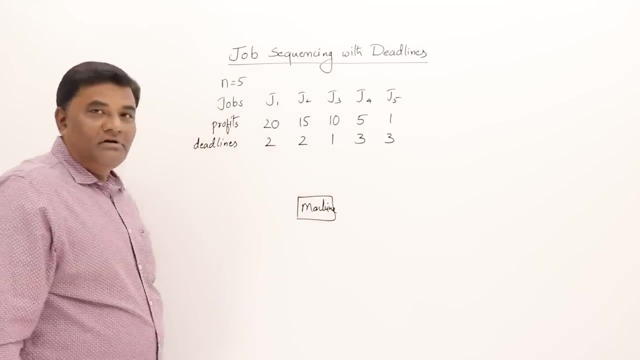 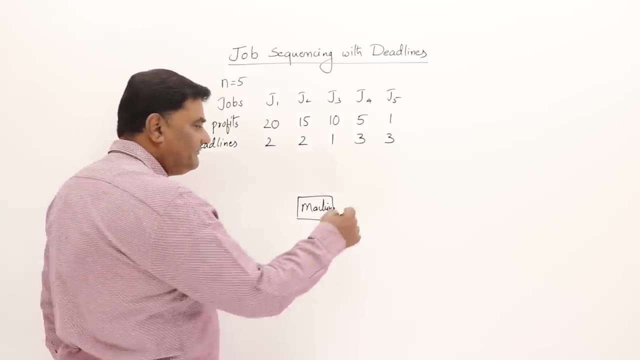 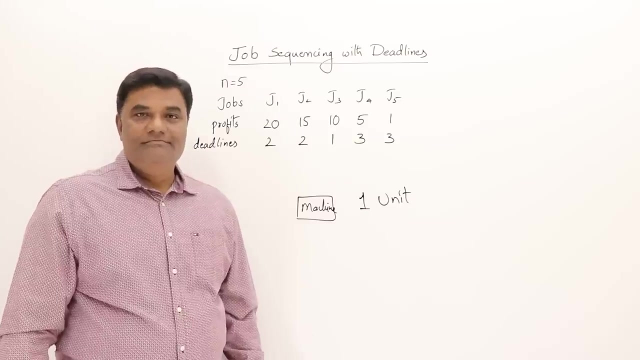 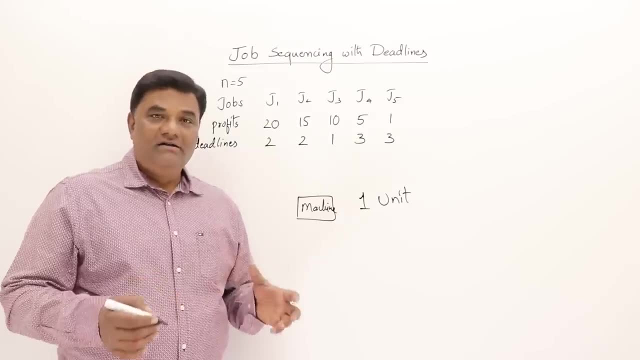 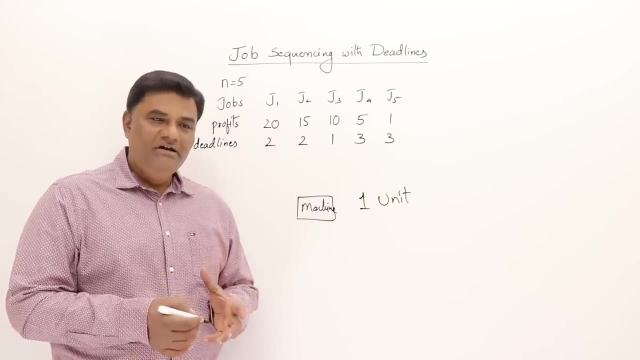 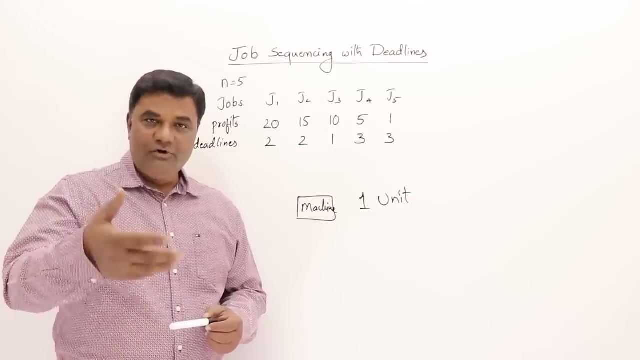 unit. I will assume this as one hour. So on a machine each job needs one hour for its completion. example, like a DTP operator or see mostly for making a legal documents for on a bond paper, we will find people in the market who will prepare documents. suppose that preparation you take the. 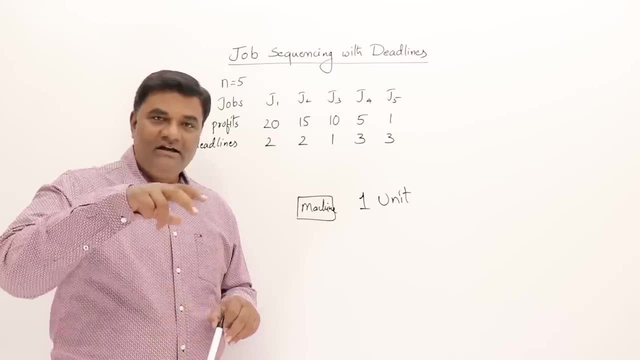 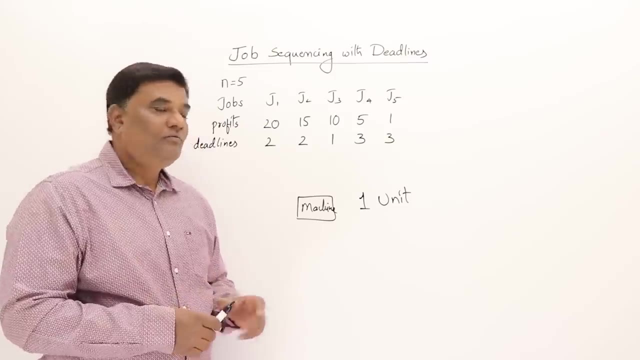 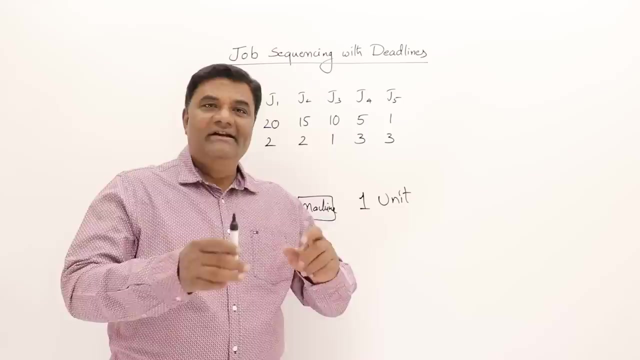 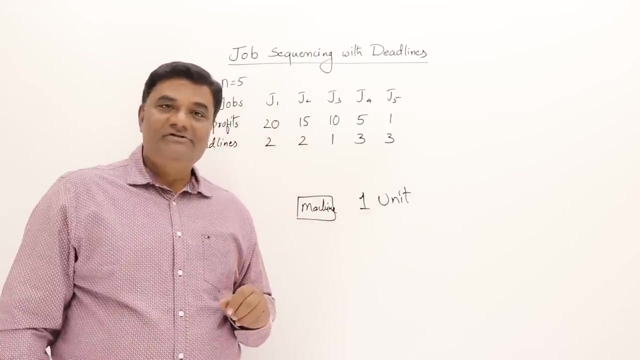 job. so he's a typist right and he completes each job in one hour. that's it. so that example you can take. now what is the situation? let us understand. see, assume that in the morning he has opened the shop, the moment he has opened the shop, these five people are standing there for getting their jobs. 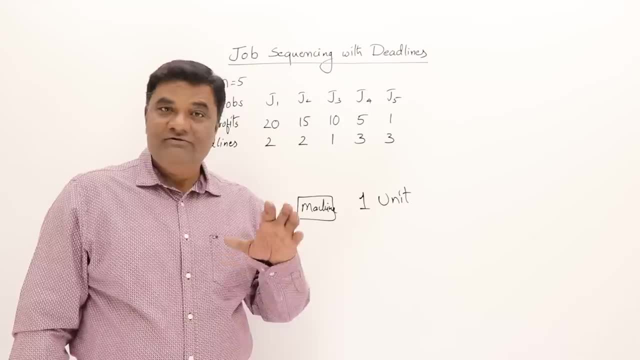 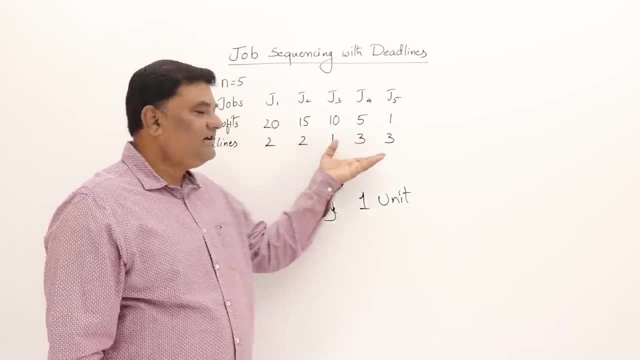 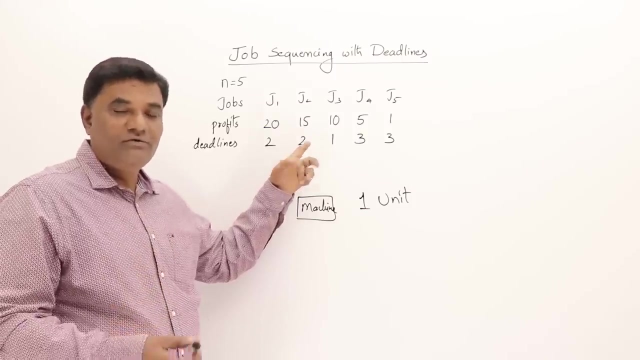 done, all right. so you have to take this situation to understand the problem, and each person is having his own deadline. he is saying that I want my job to be done first, in the first hour only can you do it or not. if you can do it, do it. and this person is: 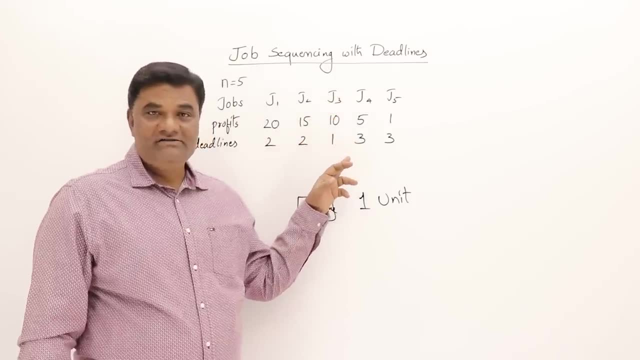 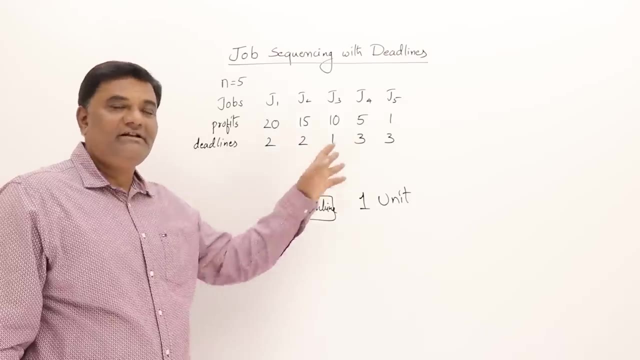 saying that I am ready to wait for three hours. no doubt my job needs only one hour, but I am ready to wait for three hours, suppose this morning 9 o'clock. so he is ready to wait till 12 o'clock and he's ready to wait till 11 o'clock, and 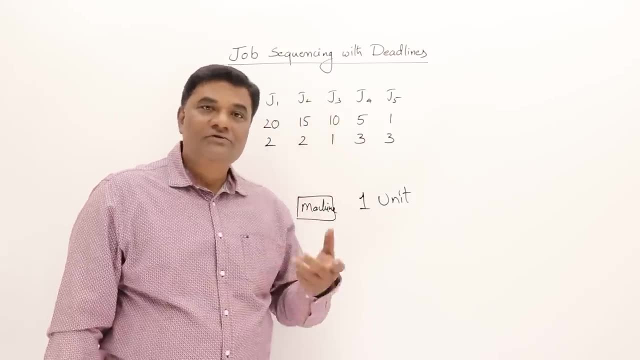 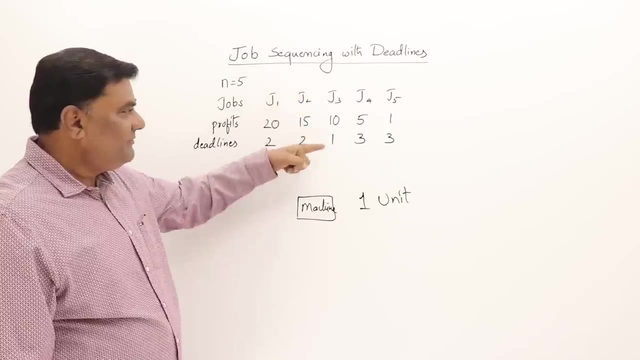 he's ready to wait till 10 o'clock. so whose job should be done first? this job should be done first. but what is the profit we are getting if this job is done? let us say this is rupees and we get just 10 rupees. and if this job is? 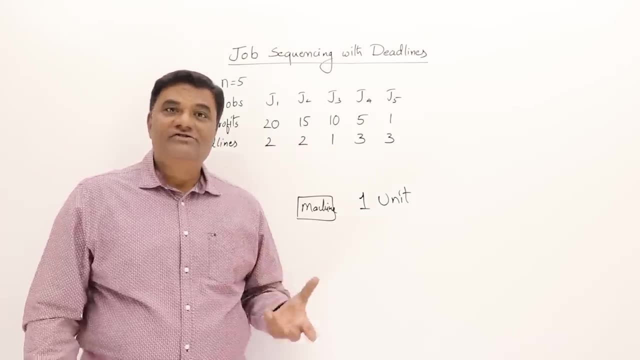 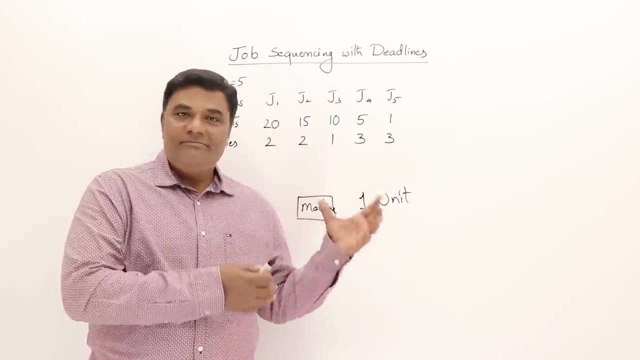 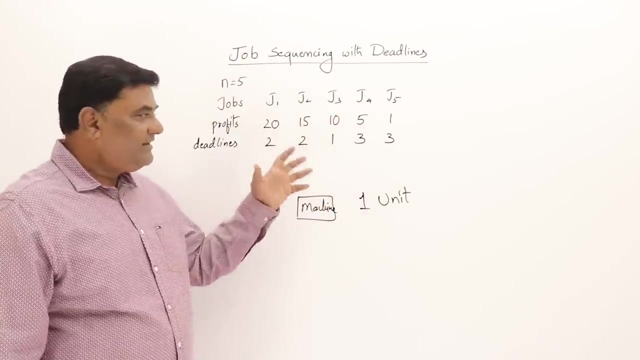 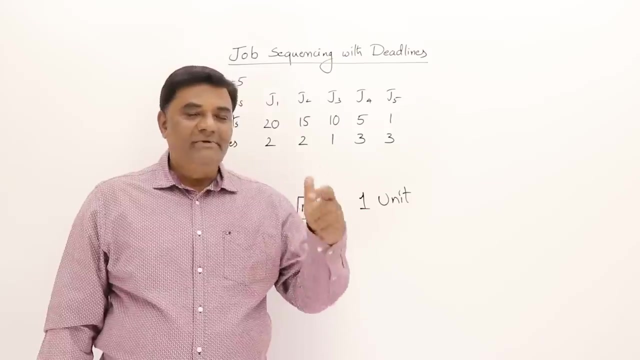 done, then we get 20 rupees. so, obviously, which job should be done first? highest profit job should be done first, yes. now the problem is, we want the set of those jobs which can be completed within their deadlines, so such that the profit is maximized. the profit is maximized, so there's a maximization problem. 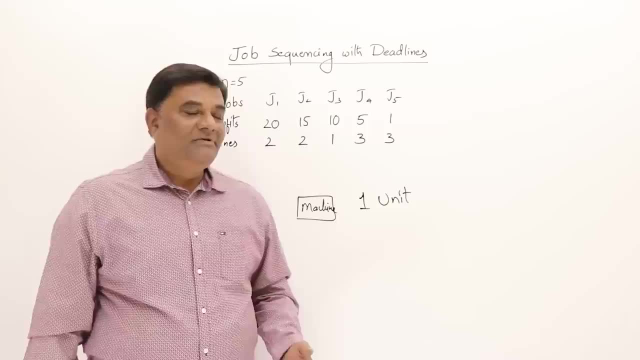 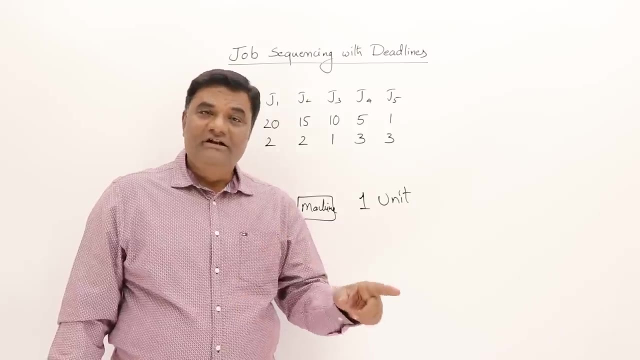 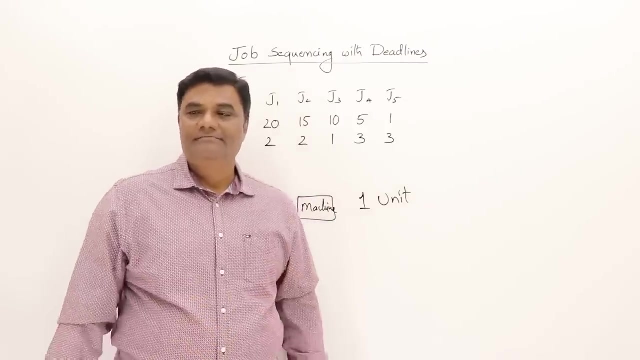 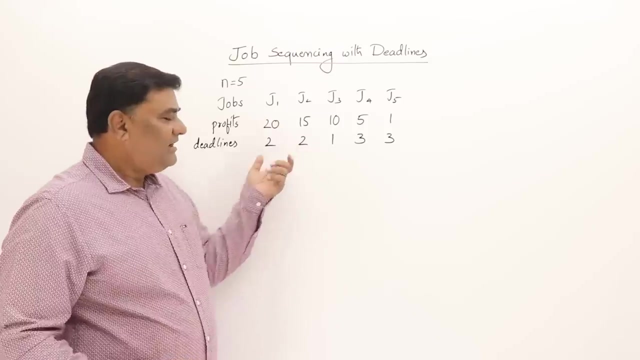 and what is the constraint in the problem? job must be completed within the deadline, all right. so this is suitable for greedy method because it's an optimization problem. it's a maximization problem, so we can apply greedy method. now let us solve this problem using greedy method. let us see how we can apply greedy method. so, first of all, how many hours are? 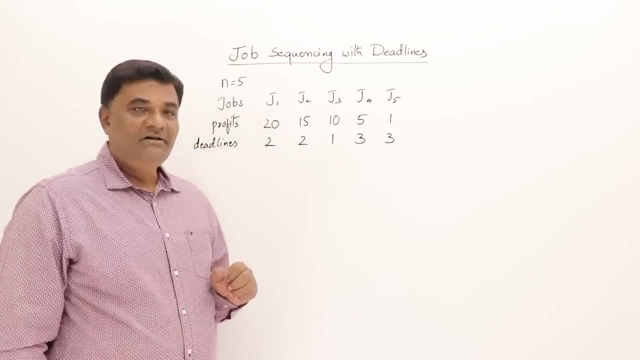 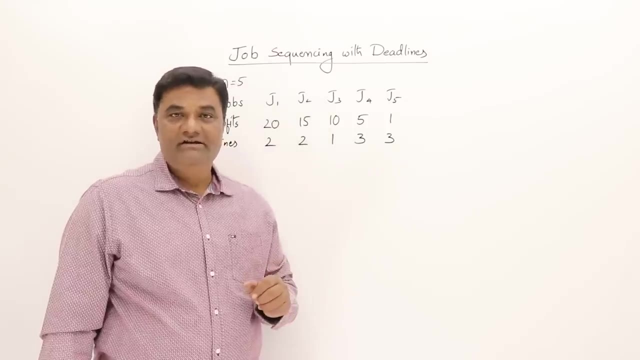 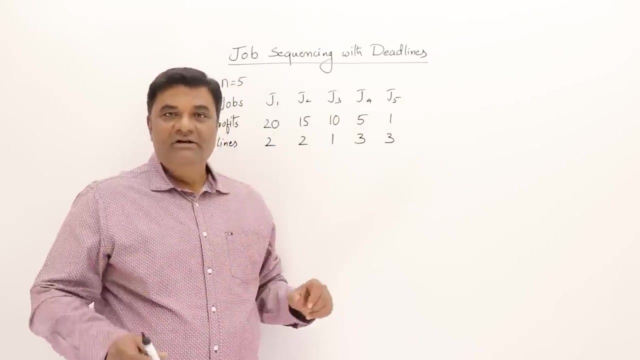 available for that typist to complete the job. see, one of the person, or two people are ready to wait till two o'clock or for three hours. they are ready to wait. so after that nobody is there. suppose this is the only job that he has when he has opened the shop and he has to complete this. 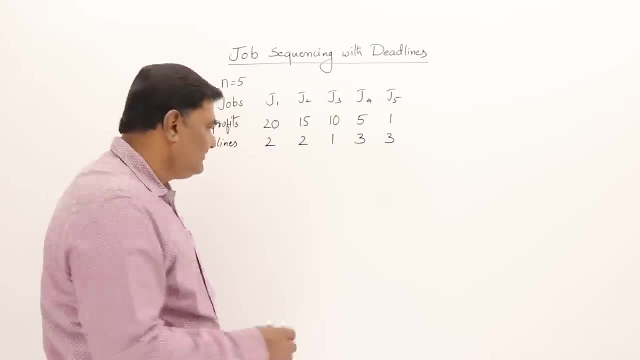 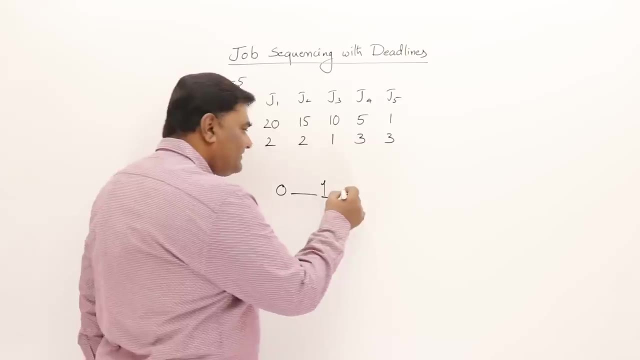 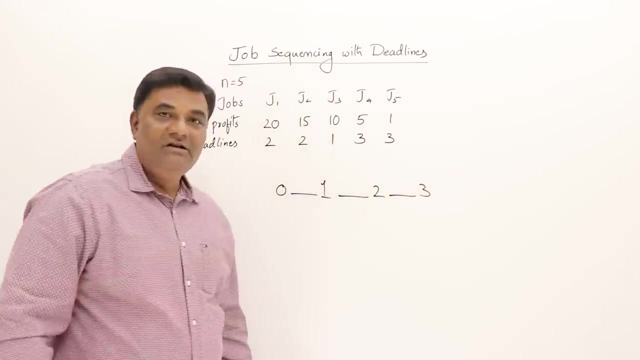 within their deadline how many slots he is having? from zero. both hour to first hour, one unit of time in this hour he can complete one job. then first hour to second hour he can complete second job. and second to third he can finish third job. so it means nobody is ready to wait beyond three units of time, three hours. so he has. 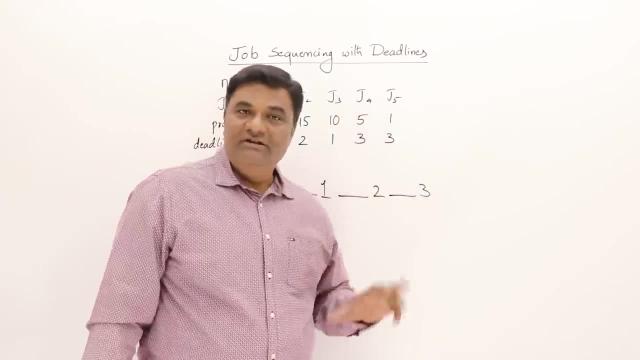 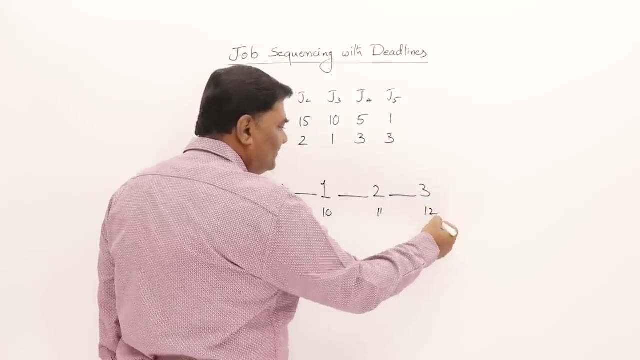 to finish jobs within these three slots only if i give the time. this is nine o'clock to ten o'clock, and this is ten o'clock to eleven o'clock, eleven to twelve o'clock. now there are only three slots. how many jobs he can do? deadlines are giving just three slots, so 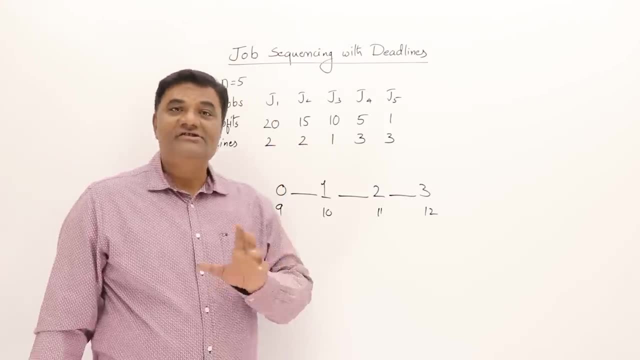 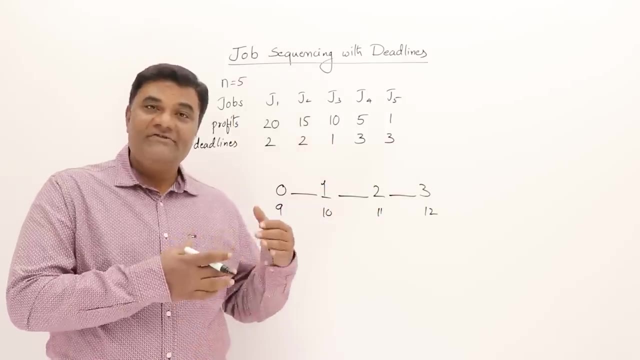 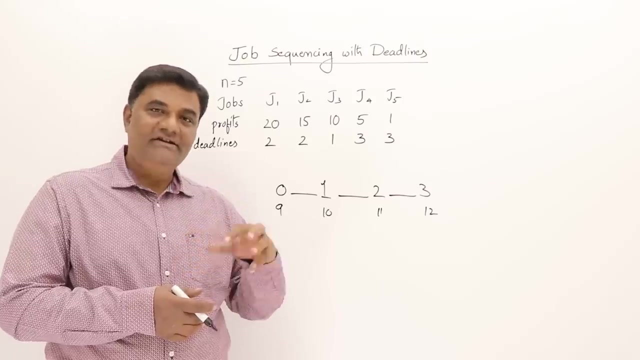 he can do only three jobs out of five. he has to select just three so that the profit is maximum. now, if we apply greedy method, then on what basis we will select the objects? we will select the objects in the order of their maximum profit. so first maximum profit, then 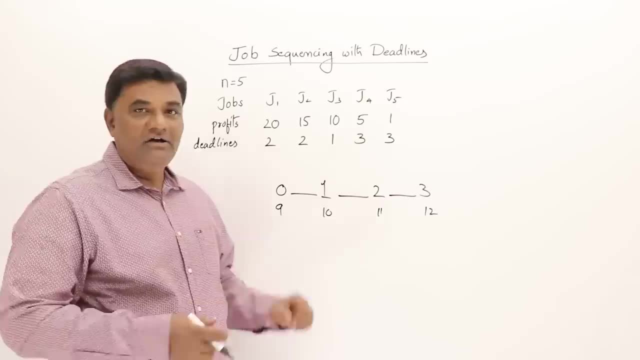 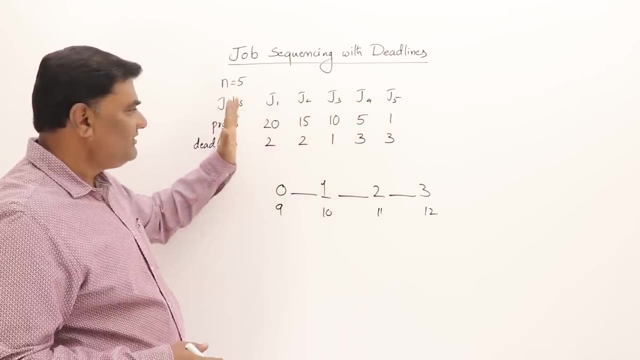 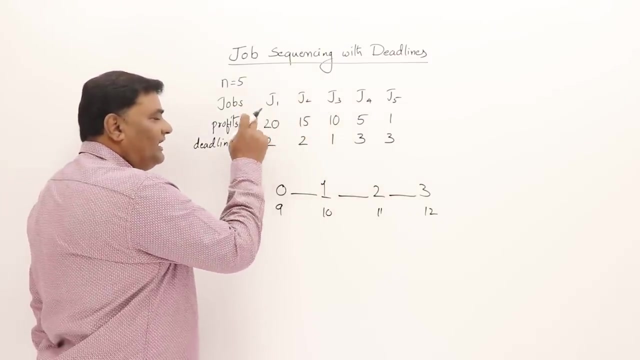 next maximum, next maximum, and so on. so let us see how to solve this one. who is having highest profit? this one. so you can see already that the jobs are already arranged in the decreasing order of the profit, so i have to consider them in the same order. this is having highest profit. now i will select. 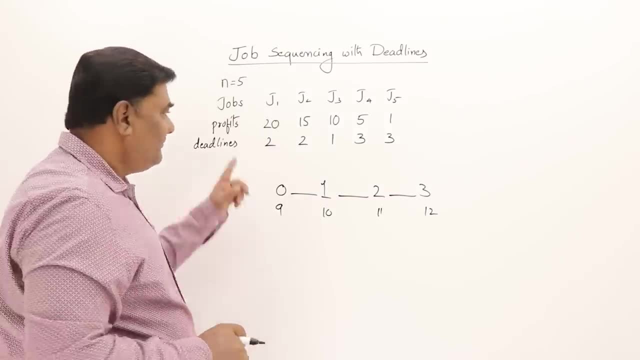 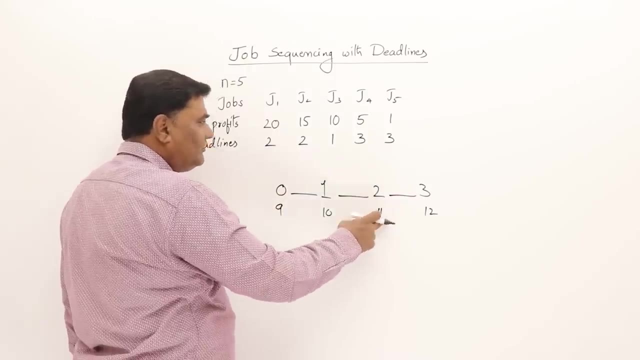 this job for completion. i will select it. i will not perform it, but in which slot i should do. he is ready to wait for two units of time, means he came at nine o'clock. he is ready to wait till eleven o'clock and his job needs only one unit of time. so let us do. 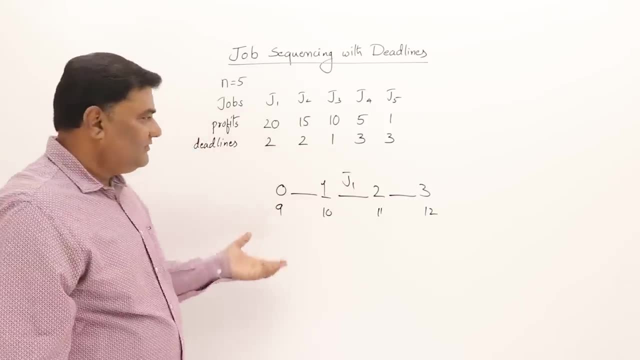 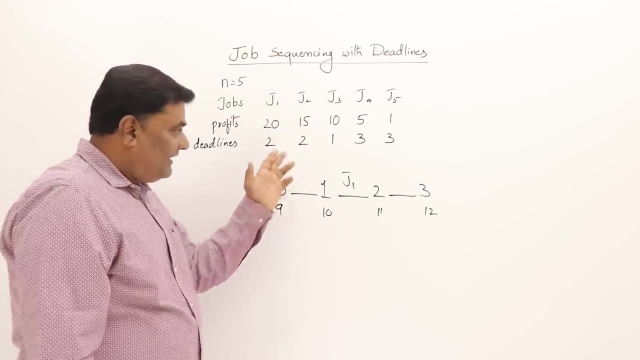 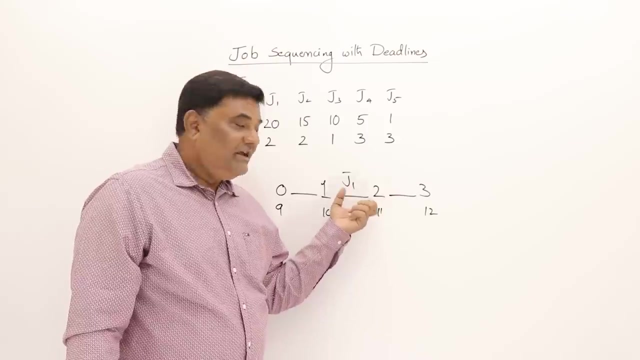 it in this slot. now let us pick up the next job. second highest profit is fifteen. and what is his deadline? two, now again go to one, to two. he is ready to wait till eleven, two units of time, but this is already occupied. now see if there are any slots available on this side. 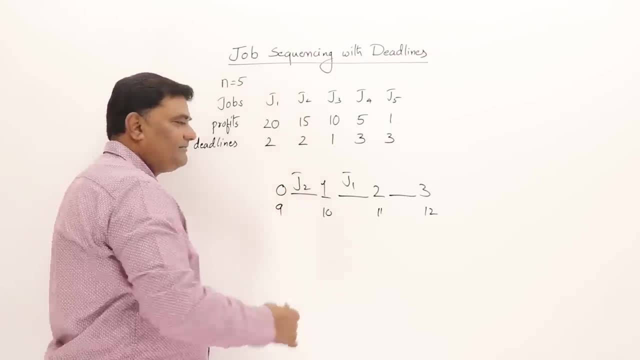 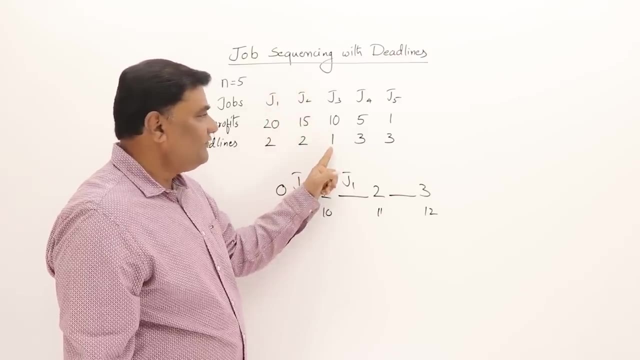 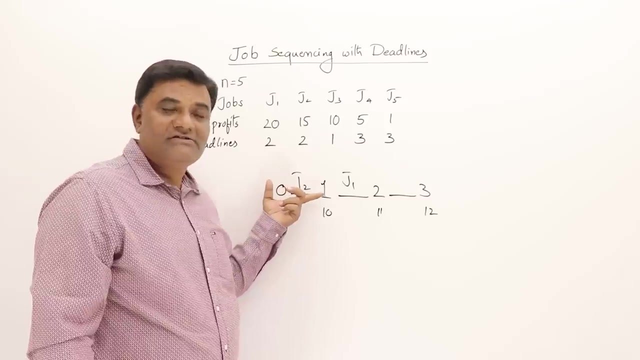 yes, it is available. so that job too, here now let us select the next job. third job: now let us select the next job. third job, third job: now let us select the next job, third job, and see if he is ready to wait till twelve o'clock and his deadline is one. can we do it? let us. 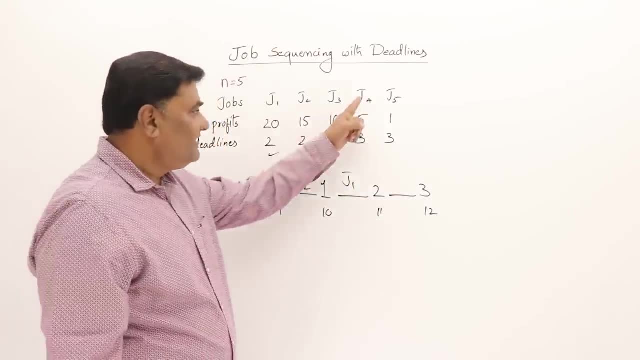 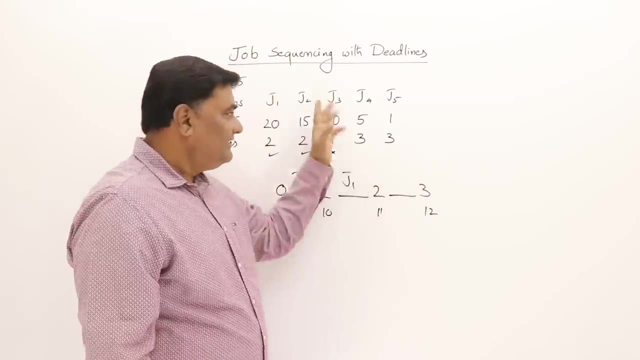 see one means what? zero to one within this one. no, this slot is already gone, so this job is rejected. we cannot do this job, so we have selected already these two jobs. then what about this job? this can be done because the deadline is three, so he is ready to wait till. 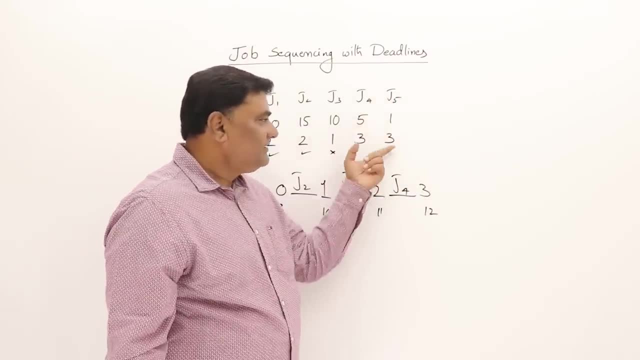 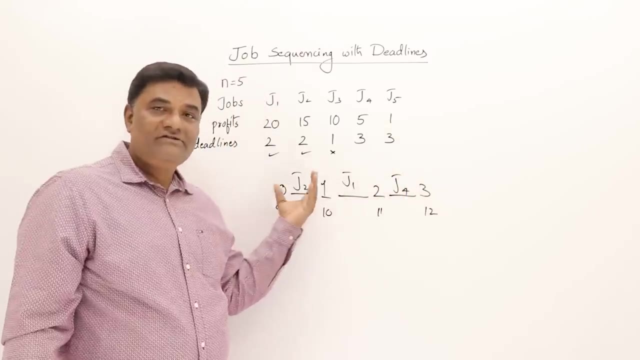 twelve o'clock or third unit, and every job needs one unit of time. remember that, so we. so that's it. and what about this job? third, already occupied. is there any slot free on this site? no, if there is no slot available there, you can look for the slots in this site. 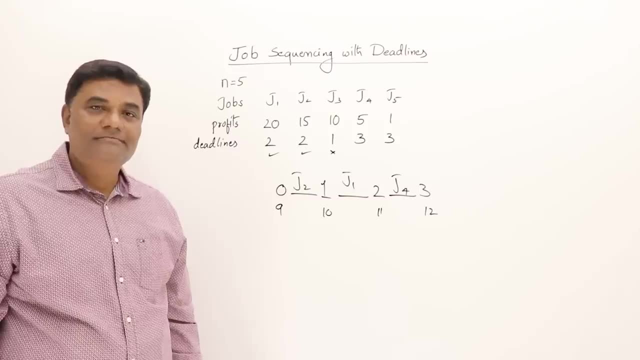 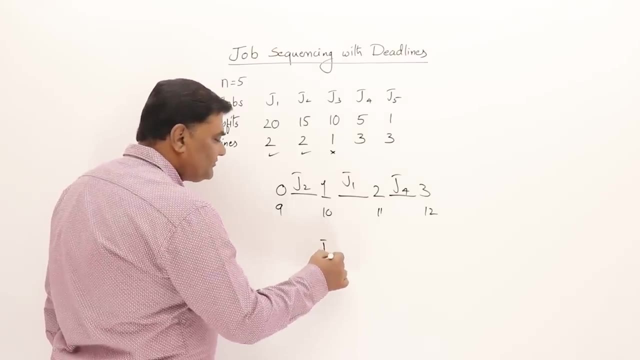 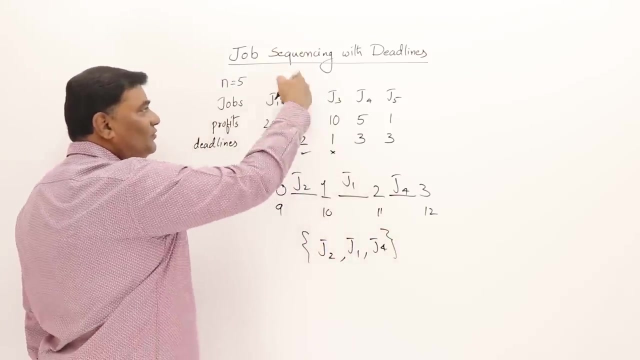 so there is no job slot available. that's all. we have a solution. what are the jobs that we are going to do? we are going to complete jobs two, then job one and job four, and in which sequence we have to do them. so here, both the jobs are having deadline two, so we can do them in sequence. 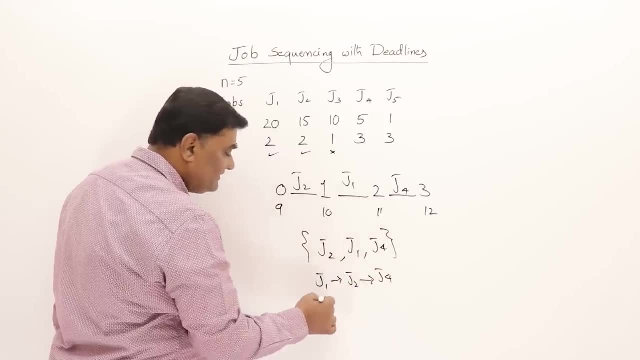 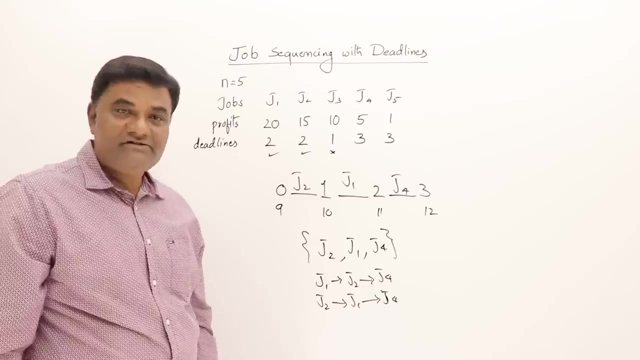 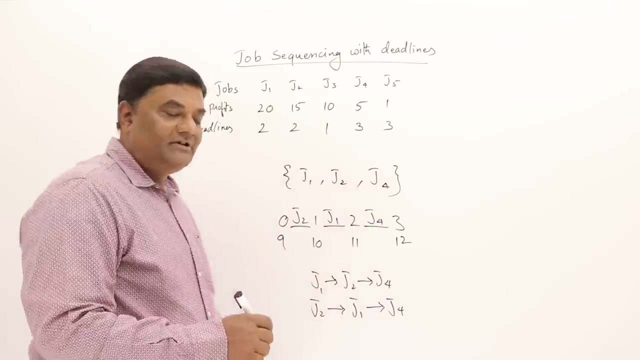 j1 then j2 then j4, or else j2 to j1 then j4. we can complete them in any of these sequences. so these are the sequences possible for completing those jobs. as both are ready to wait for two hours, total profit will be: this job is 20 and this job is 15, and the profit of this 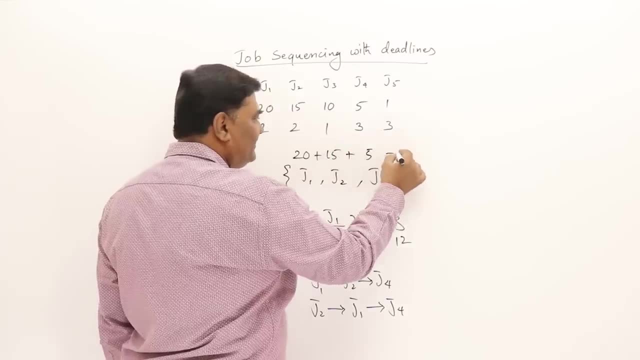 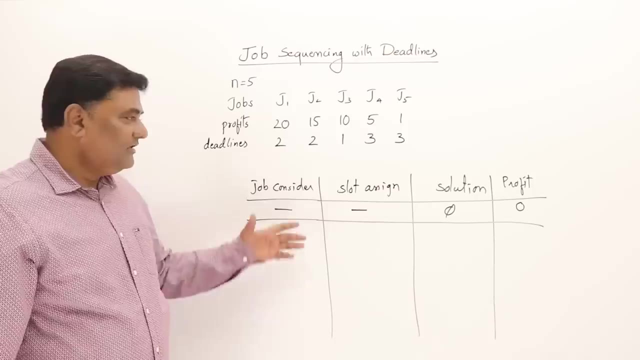 job is 20.. is 5? so it is 20 plus 15 plus 5 is 40, so the total profit that we gain will be 40. now let us solve this here. i have a taken table now. initially, there is nothing and there is nothing in the solution. 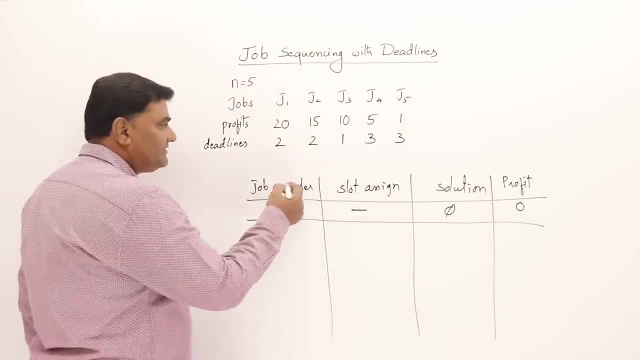 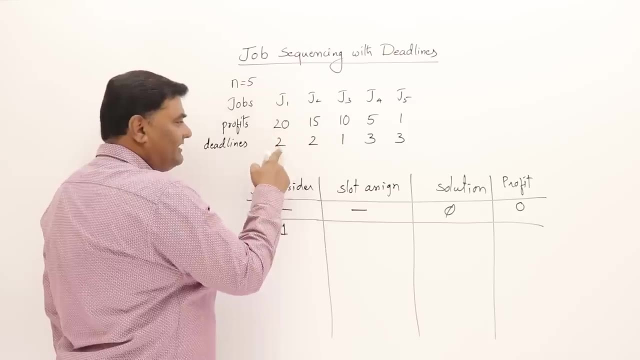 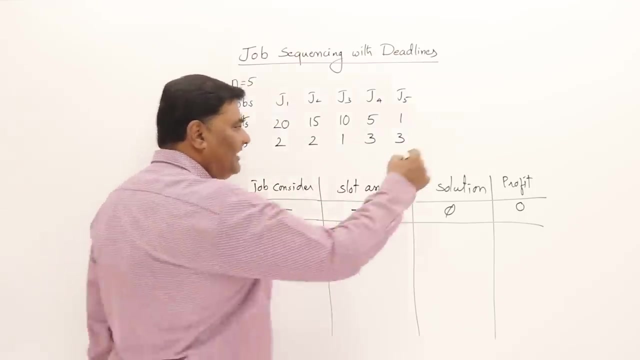 and the profit is also zero. let us start first which job we will consider job to be considered. first job i'll write 1 or j1. first job i am considering and first job, as the red line is 2, we will assign a slot from 1 to 2, 1 to 2. you remember, we have the slots from 0 to 1 and 1 to 2. 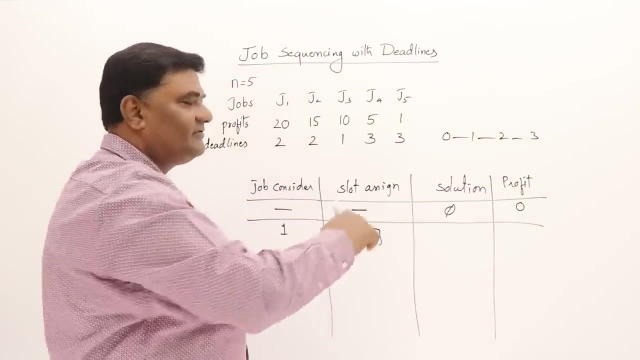 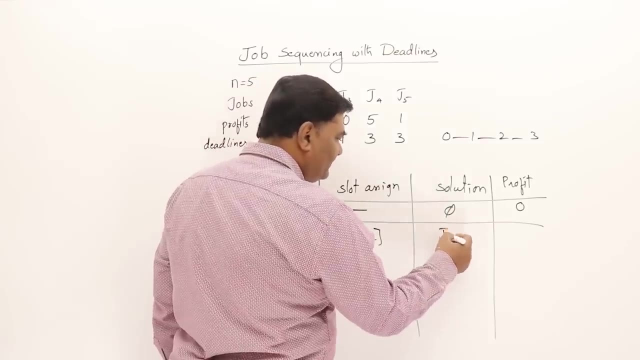 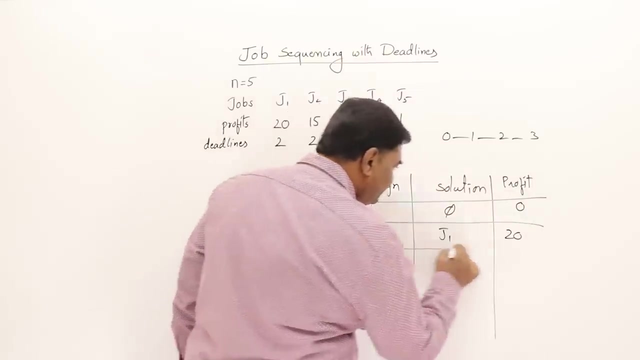 and 2 to 3, because the maximum deadline is 3 here. so these are the slots available now. solution: as this is included, we have allotted this slot job 1 comes into the solution and what is the profit? 20 is the profit. so this first job is included. then consider second job. 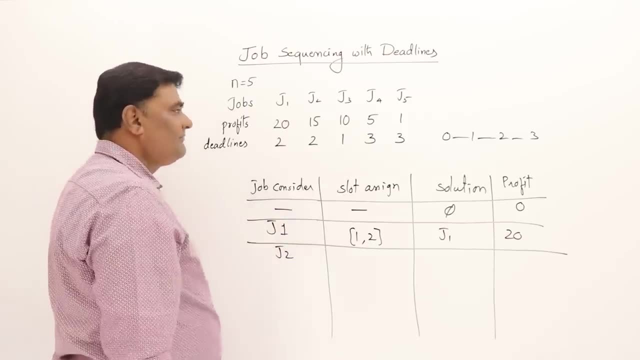 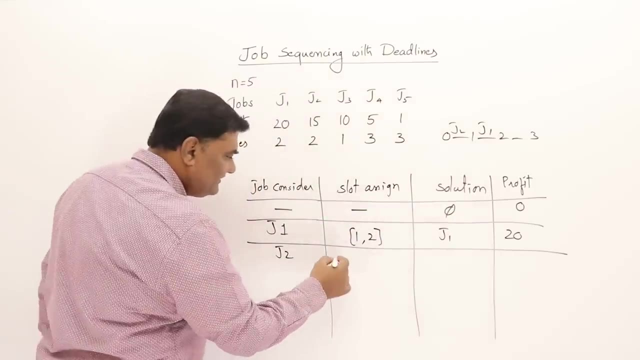 okay, j1, i'll write j2. can you assign a slot to this second job, like j1 was here? yes, j2 can come here, so we will assign a slot from 0 to 1, and already 1 to 2 was already assigned to this one. 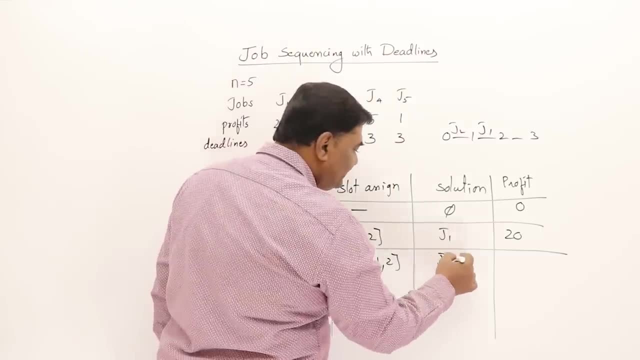 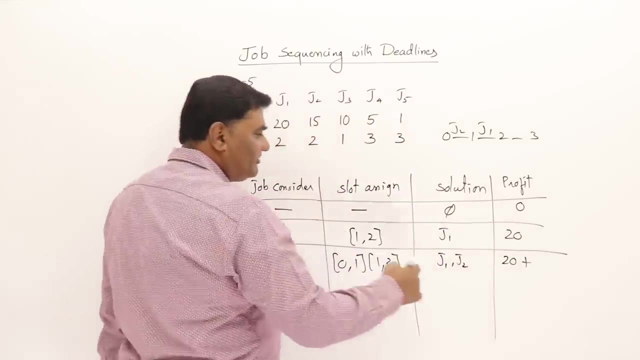 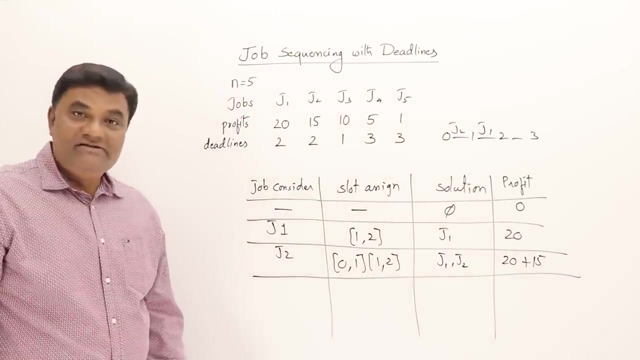 so already two slots are over, you see, and we have the solution: j1 and j2. how much profit we have? 20 plus the profit of the second job is 15, so this is 35. i'm just keeping it as it is now next job to be considered, j3, third job, its deadline. 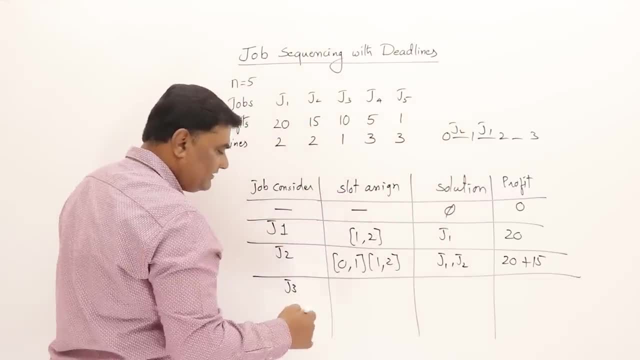 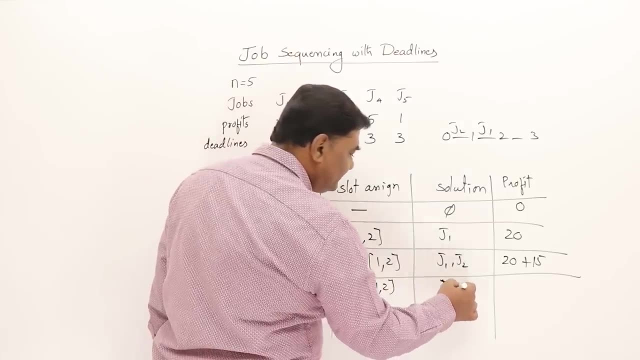 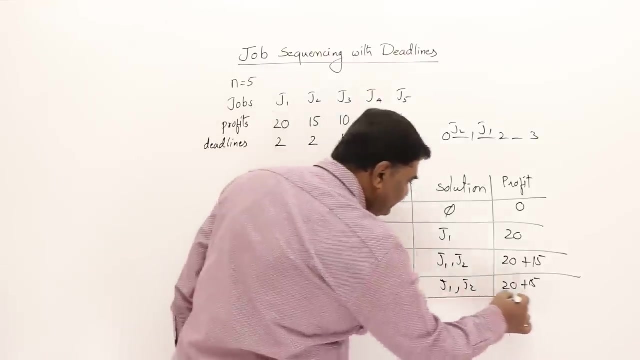 is 1: 0 to 1 all the day occupied, so no slot is assigned and everything remains the same, and jobs are j1 and j2 only, and this is 20 plus 15 only. so this job s not included in the solution. now next. 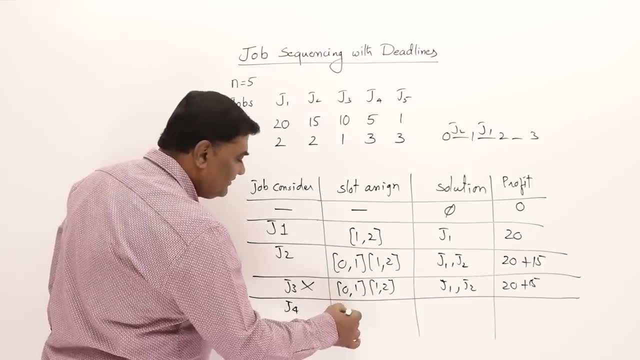 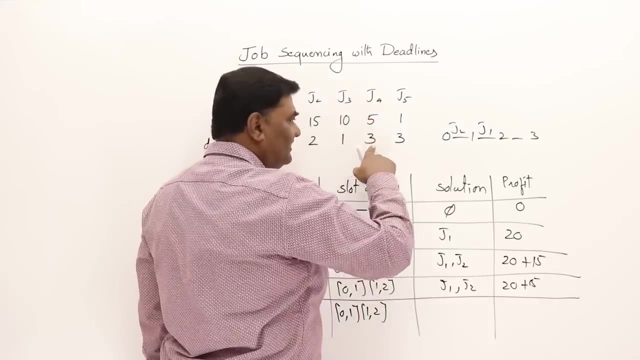 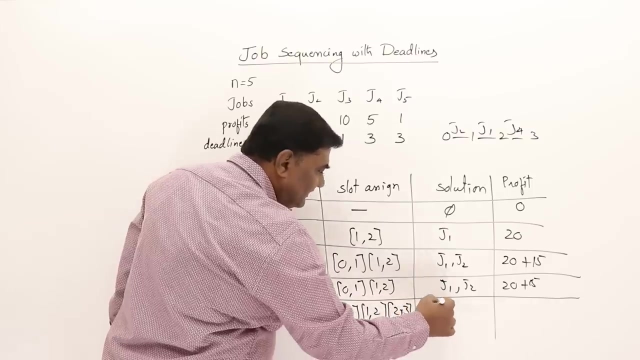 J4, so we can assign a slot. 0 to 1 is already gone. 1 to 2 is already gone. J4 can be done in slot 2 to 3, so this is J4, so here we have 2 to 3 and the solution is having J1, J2.. 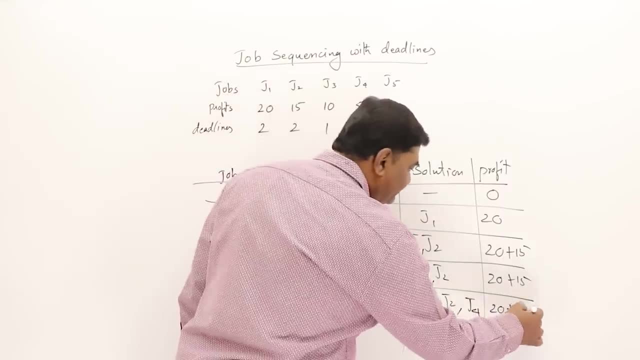 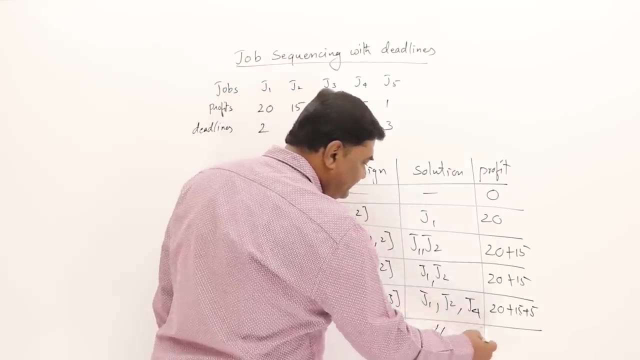 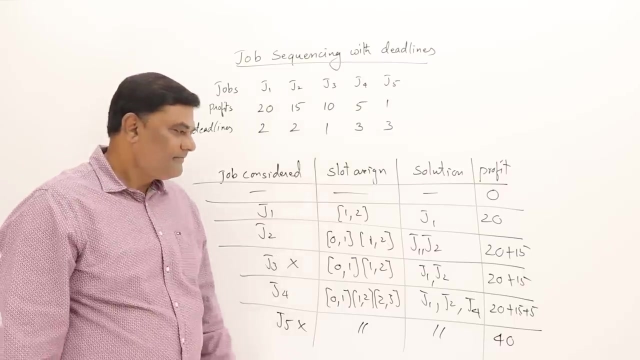 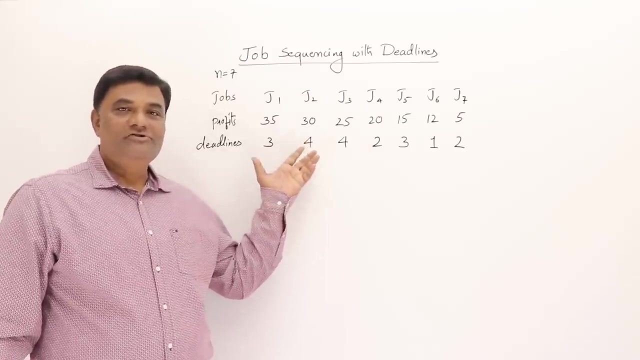 J4 is selected and it is 5 and J5, it cannot be selected. so this remains same, this remains same and this total will be 40,. total will be 40.. I have taken one more problem for solving this using greedy method. it's a problem for job sequencing with deadlines. we have to follow greedy method. 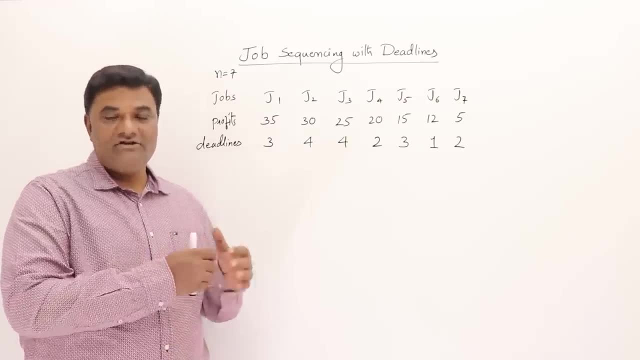 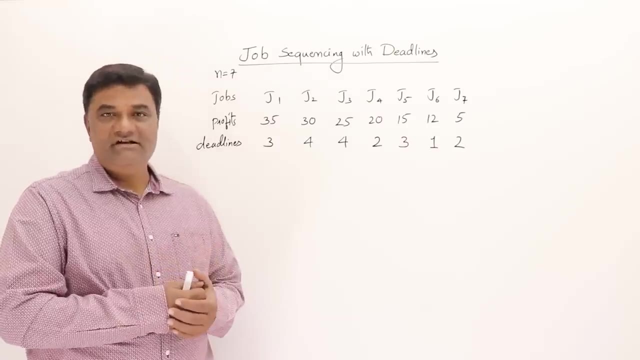 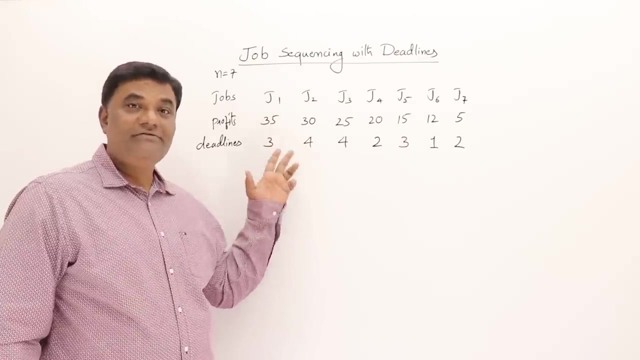 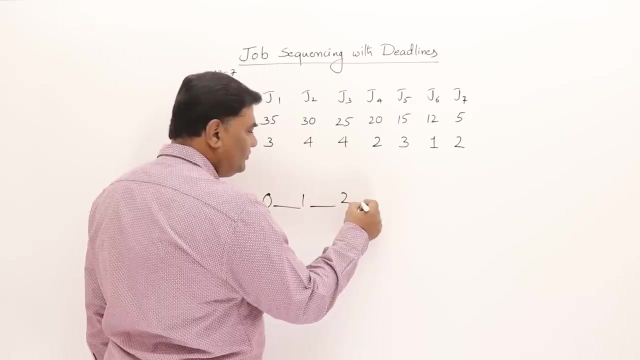 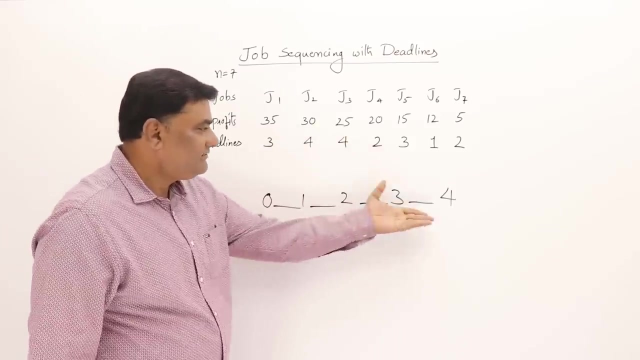 So we decided that we will select the job. We will select the jobs in the decreasing order of their profits, and that's how we may be getting maximum profit. but the constraint is they have to be finished in a deadline. so how many deadlines are there here? what is the maximum time we have to submit any job? maximum time a job can be submitted is 4, so how many slots are available? 0 to 1,, then 1 to 2,, 2 to 3,, 3 to 4, maximum deadline: 4.. 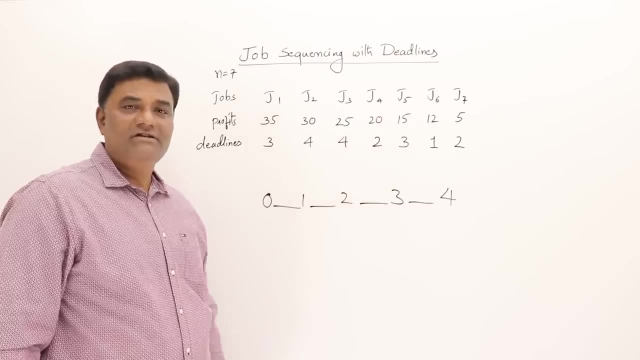 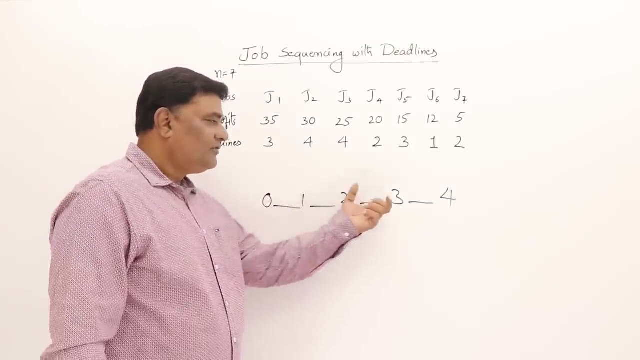 After that, nobody is ready to wait. the job should be completed within that 4 units of time, but every job needs just 1 unit of time. so how many slots we have with 1, 1 unit? 4 slots we have.